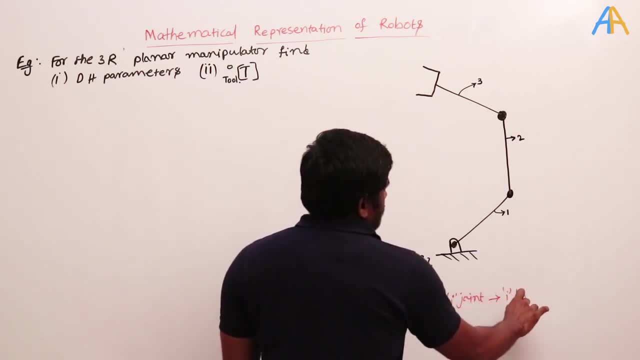 and then I link. I mean I link. So first link, First link, means before first link, first joint should come, So it will become Z1.. Okay, and here it will become Z2, and here it will become Z3.. 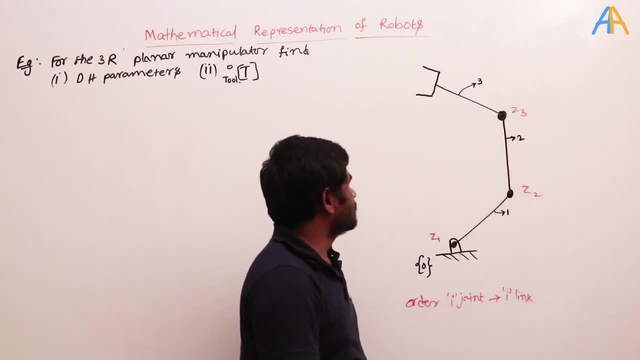 Okay, so we have Z1,, Z2, Z3, and so far we have these, and here the joint between the first link and the fixed link is the rotational joint. So whenever there is a rotational joint, then what are the condition that I told You need to choose the coordinate axis of the fixed one and then 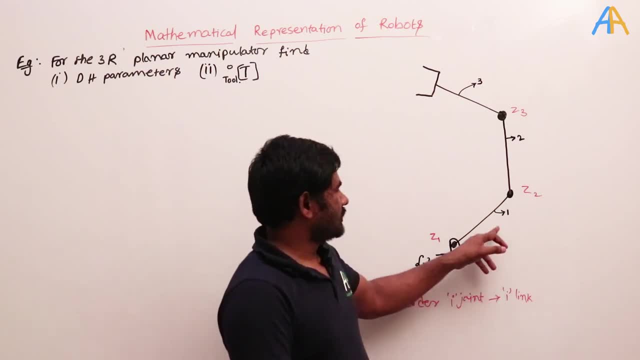 the immediate Z1, immediate first link joint, that is Z1, in such a way that both are coincident. So here we have Z0.. See this: Z1,, Z2, all these are coming out of the plane. Okay, the rotation. 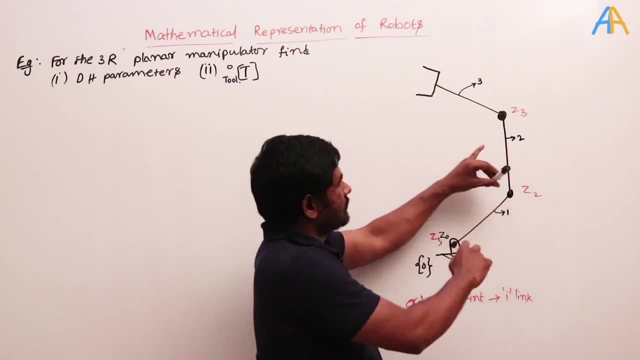 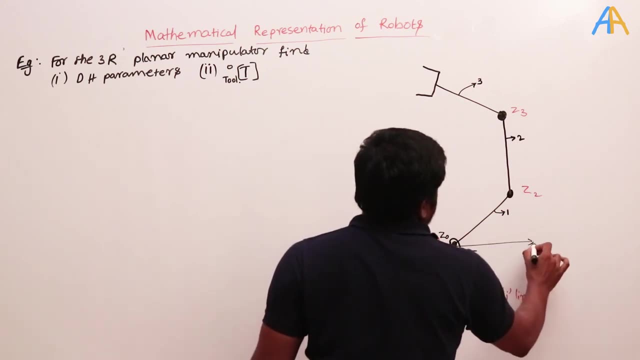 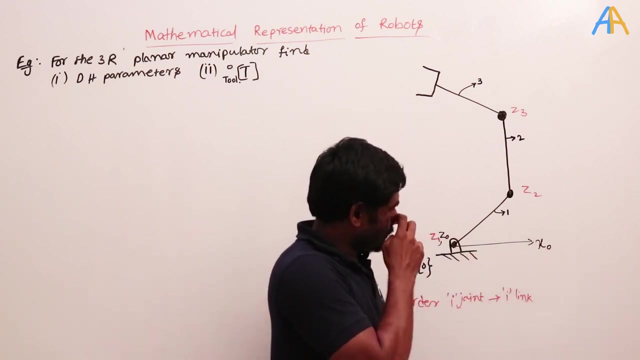 it is rotary joint is like this: They are rotating about this. So when I rotate like this, it is coming out of this and I will choose the X0 arbitrarily. Okay, this is a X0.. This is X0 and this is a Z0.. So we found out the Z1, Z2, Z3, and now we are. 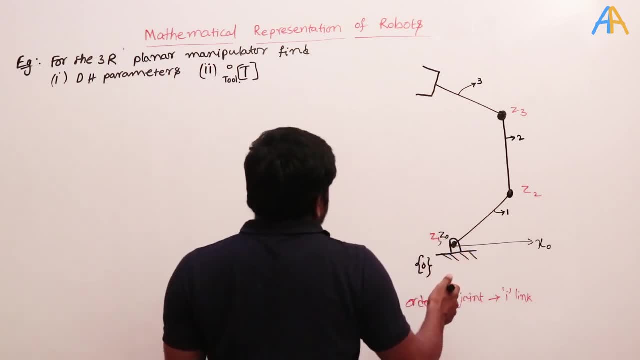 otherwise, we can find out Z1,, Z2, Z3 in another way also. What is that? To find out the L1. L1 is nothing but Z1. It is the between, the you know 0 and 1, links between 0 and 1.. Okay, L2 is between: 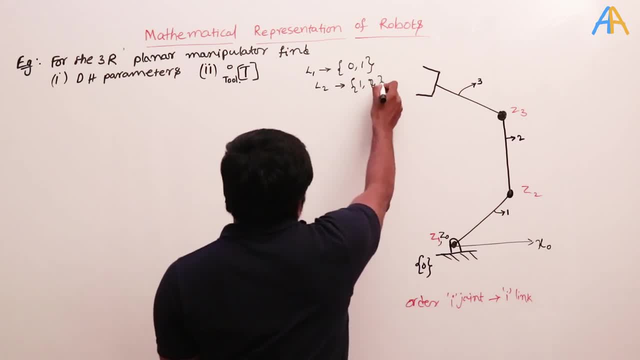 the 1 and 2, 1 and 2, links between 1 and 2.. Okay, like that we need to find out. And now we need to find out. the X, X, I we need to find out from. XI is the distance between. you know, XI is the distance between. 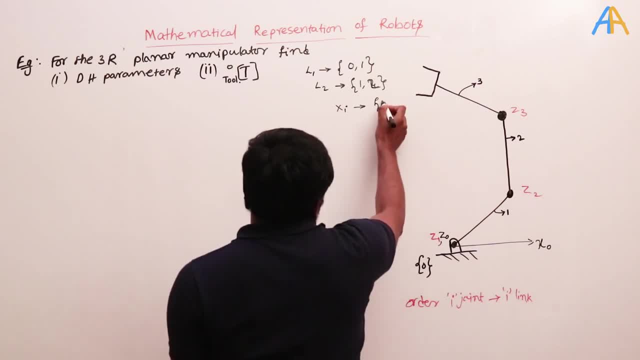 what It is, the distance between ZI, ZI plus 1.. Okay, ZI and ZI plus 1.. So here, in this case, for example, I will take something like a X0 is already found out, X1,, X2,. 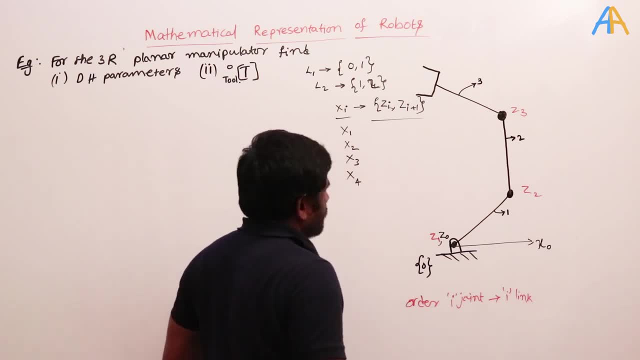 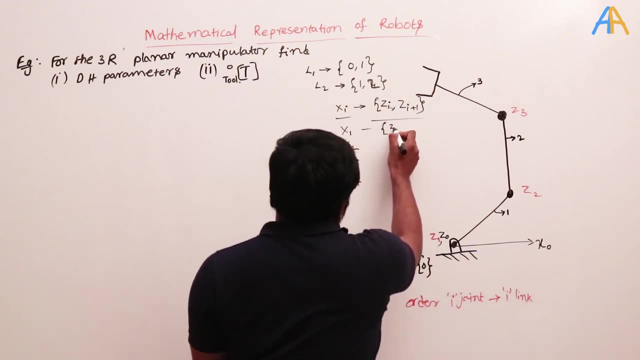 X3 and then X4. So I need to find out this. So for that I need to have here what is that? Z1, Z2.. For this Z2, Z3 and for this Z3, Z4.. Okay, so we don't have Z4 here. We have. we have only. 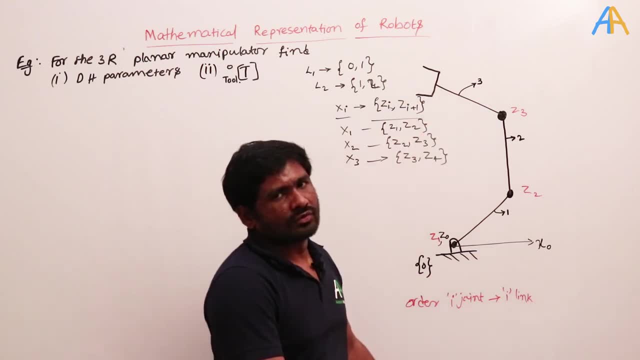 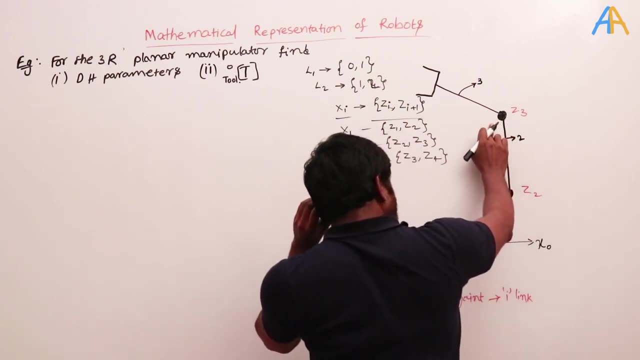 chose of the end effector at the tool, At the end of the tool. Okay, So whenever there is a, if the Rth joint is a, if the Rth joint is a rotation, then we can chose either the last two tool coordinates: is, is a, is a coincident or something along the parallel. So I have 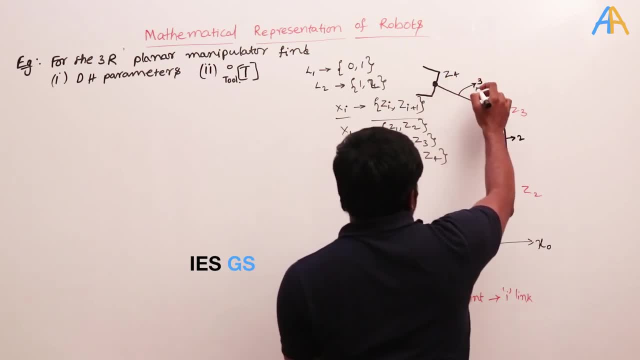 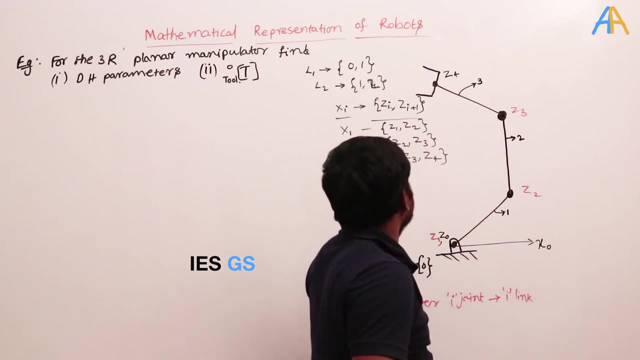 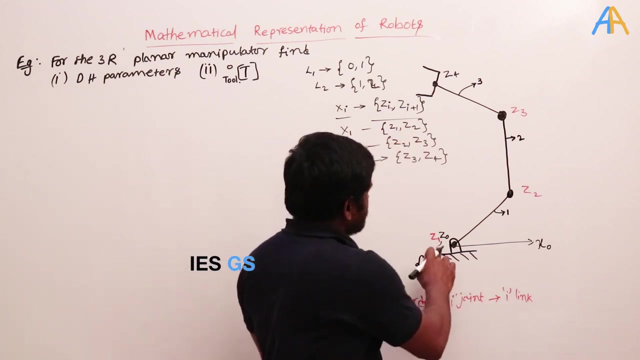 chosen here. This is a Z 4.. I have chosen the Z 4 in a such a way that it is coming out of this plane. Okay, it is coming out of the plane. So here we need to find out first, x1. x1 is a perpendicular distance between z1 and z2. this is a z1 and this is a z2. 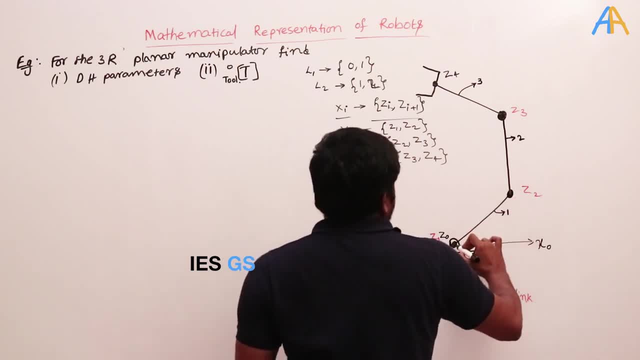 the perpendicular distance between these two is nothing, but in the plane is the line joining these two. so the x1 is like this x1 is like this, okay. and since it is a rotary joint, we have a angle, theta 1. here i will say this is the length l1, and this is the l2 and this is the l3, okay. 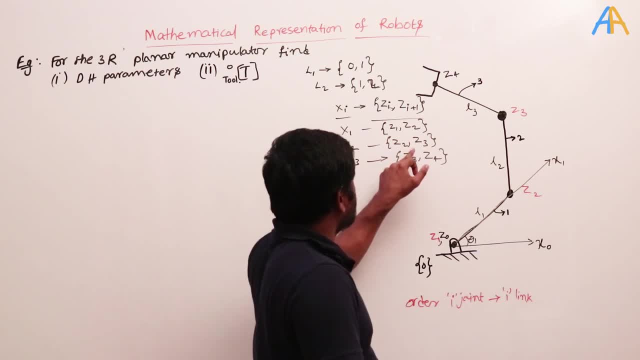 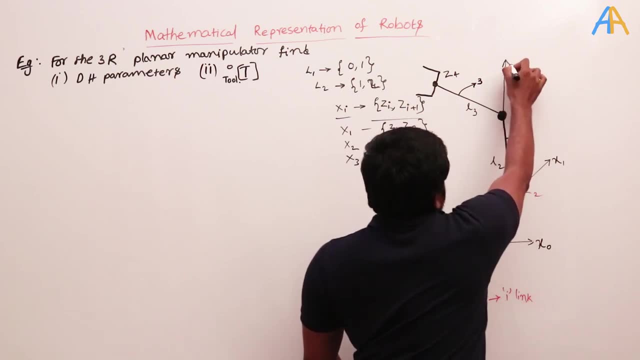 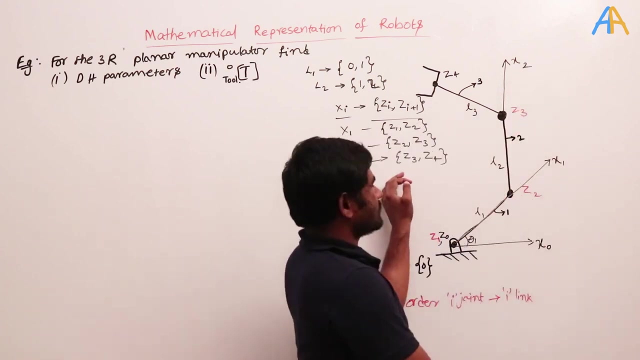 so and in the same way, x2. x2 is the perpendicular distance between the z2 and z3, so it is a perpendicular distance between z2 and z3. so x2 and again x3. x3 is a perpendicular distance between a z3 and z4. this is z3 and this is the z4. both are, you know, coming out of the. 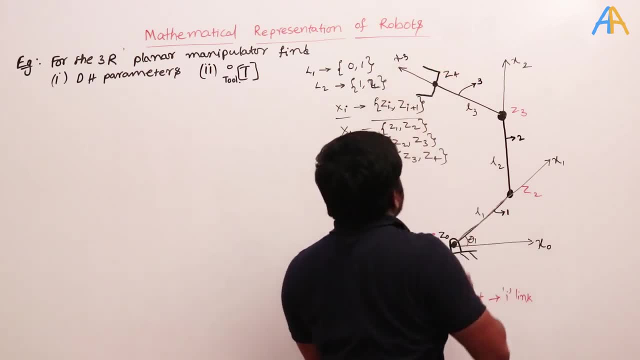 paper. so this is the x3. okay, so here i will choose the exit tool, also exit tool, you know- along the x3. if i choose x3, x2 along the s3, then what happened? the theta value, it will become 0 at the end. okay, so i have chosen like: 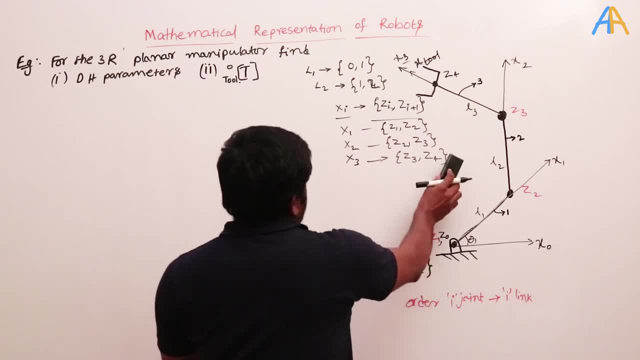 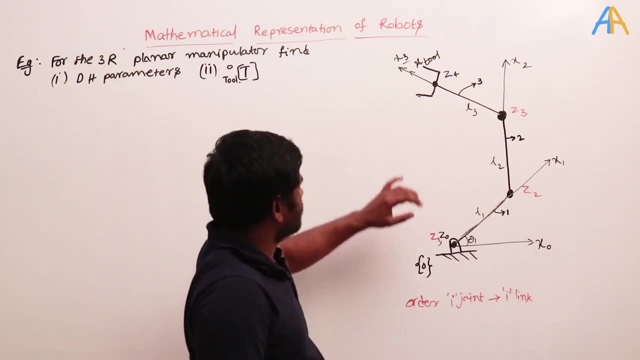 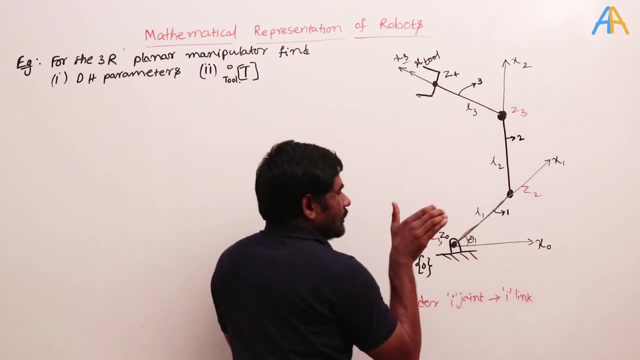 that. so here, so far what i did. i'm arising this. so so far what i did. i uh, i noted down, you know, coordinate axis. so here the z is coming like this and x is going like this. so right hand thumb rule: from z to x, z naught to x, naught. if i go like this, then this is a. 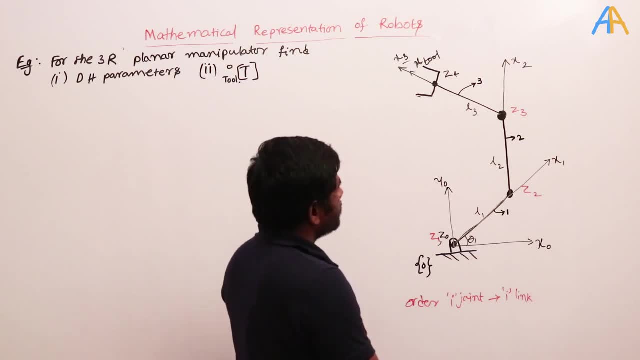 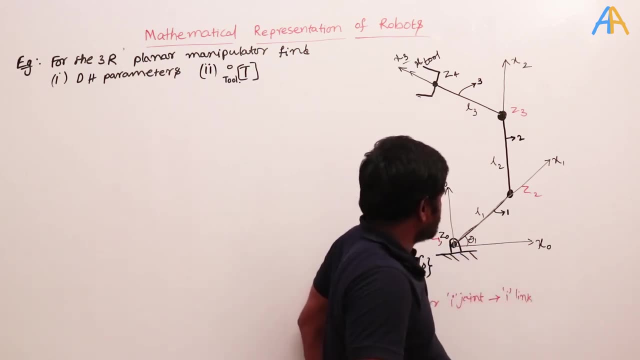 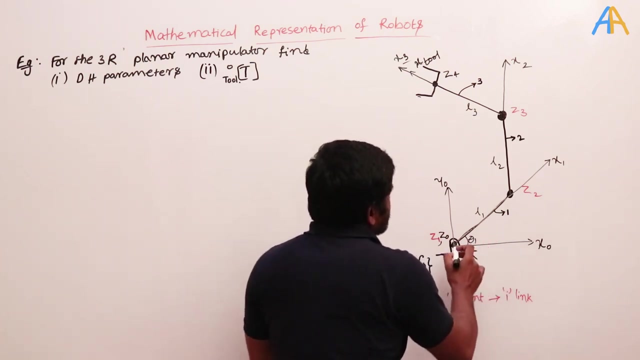 you know y naught, okay. so now i identified all the um, all the values, and here theta 1 is the angle between. actually, the theta 1 is angle between x i minus 1. that means x naught and x 1 along the z1, okay, along the z1. and here it is the theta 2, and here it is the theta 3, okay, 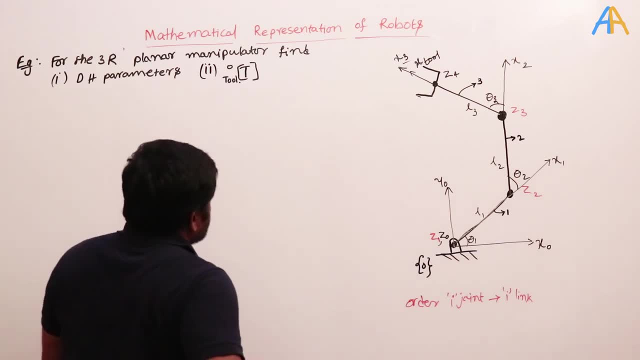 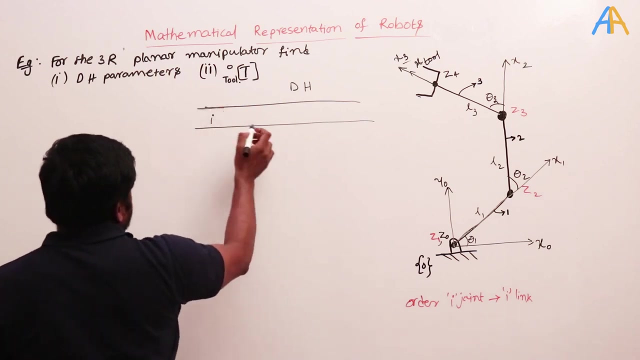 it is the theta 3.. so here we need to find out the first dh parameters. okay, i will write the dh parameters table. so dh parameter. so how many parameters are there? first of all, four parameters are the? how many links are there? three links are there. 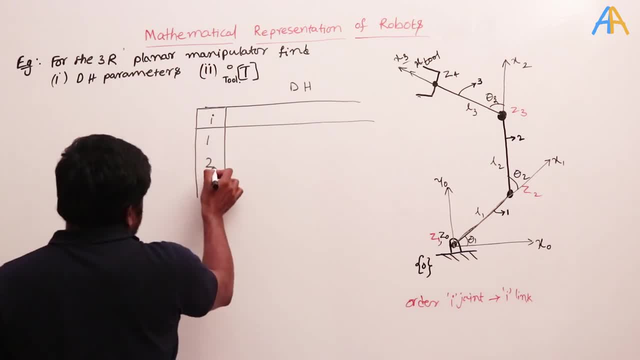 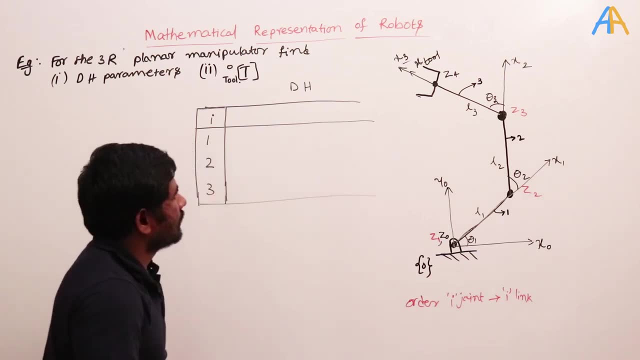 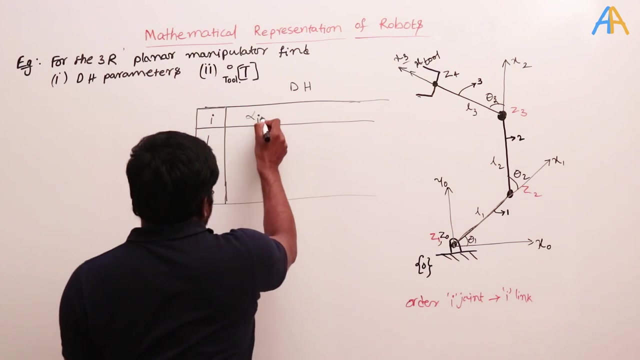 three links are there. so one, i equal to one, i equal to two, i equal to three. three links are there, okay, so what is happening here? what are the parameters? different parameters. okay, this is the alpha: i minus one. one parameter. a, i minus one, and then d i. 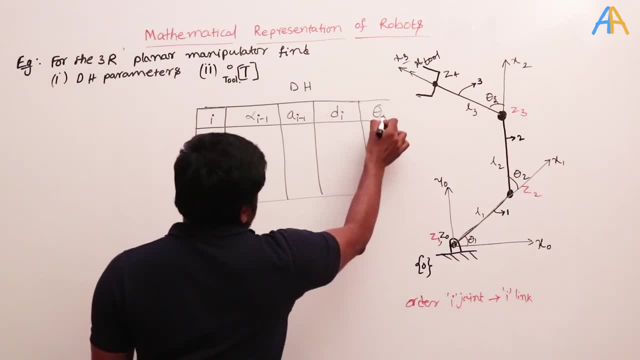 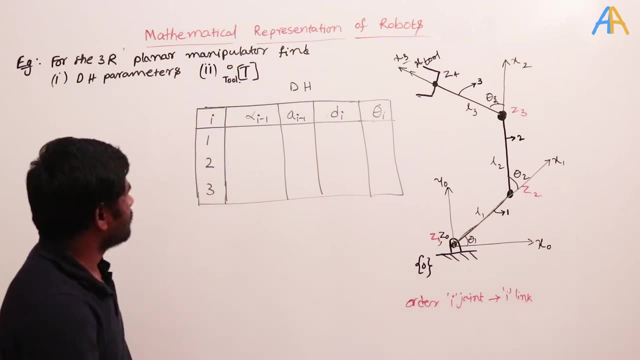 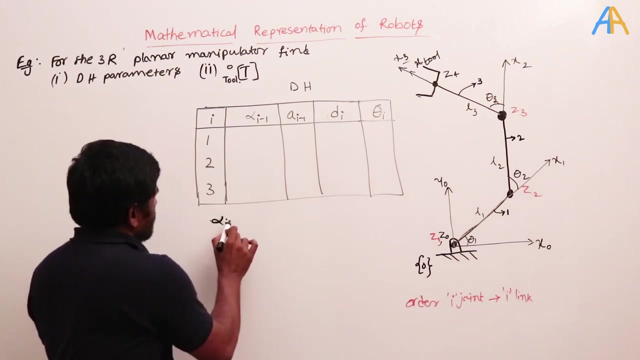 and then theta i. so by this time you should remember each and everything, okay? so what is the alpha i minus one? see, for example, if i write for alpha i minus 1. alpha, if i write for alpha i minus 1 here. so alpha i minus 1, alpha i minus 1 is nothing but the angle between z i minus 1. 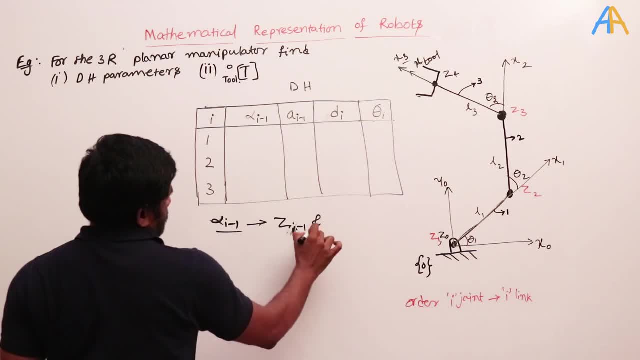 z i minus 1 and z i okay. this is the angle between this. these two a about x i minus one. okay. for example, if i put x equal to one, so that means, um sorry, i equal to one, then it will become alpha naught. alpha naught is between the: 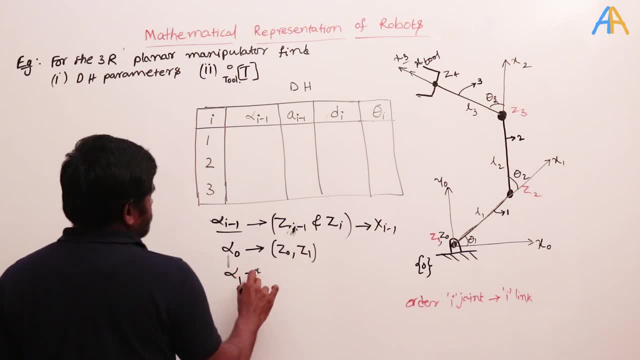 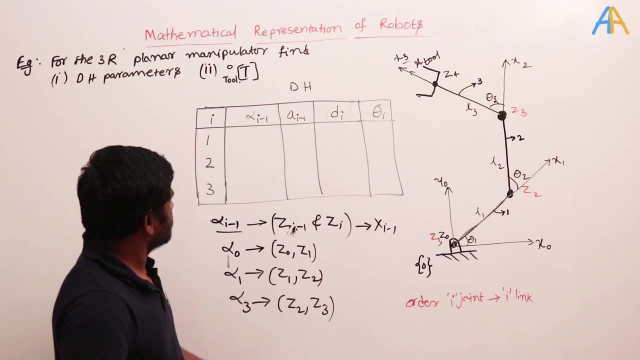 z naught and z 1 and alpha 1 is between z 1 comma, z2 and alpha 3 is between gm1 comma and alpha 3 is between z 2 comma, z 3. okay, so here if i find out the you know for the link one, if the angle. 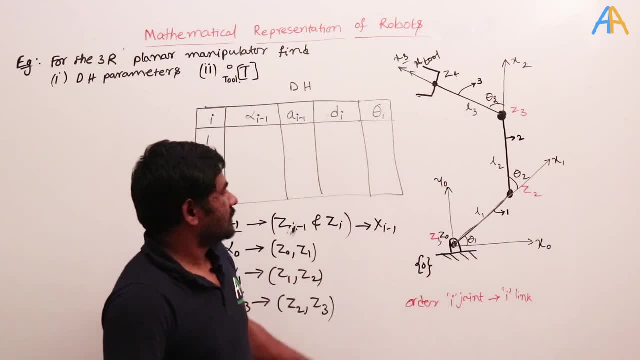 between z naught and z 1. the angle between z naught and z 1 is a 0, why? because the both are coincident, okay, and alpha 1: that is the angle between z 1 and z 2. so where is the z 1? here z 1, and what is the z 2? that is the z 2, okay, so this is the again the angle. 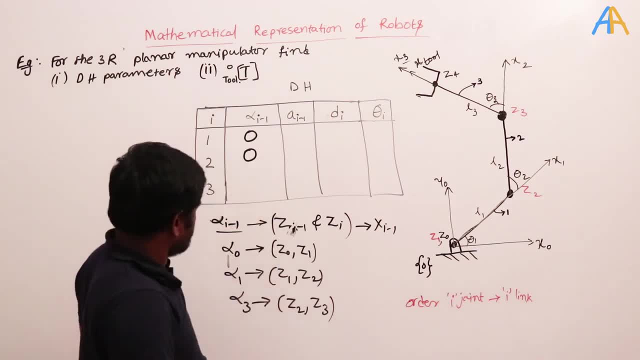 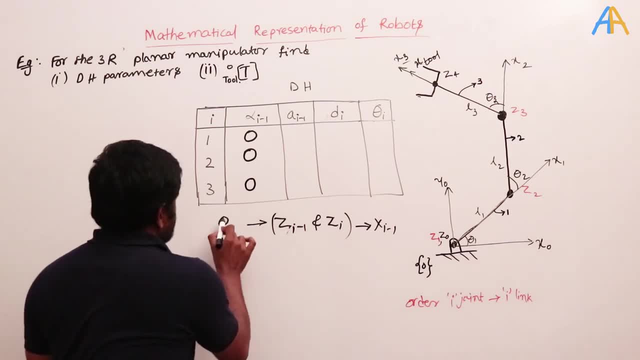 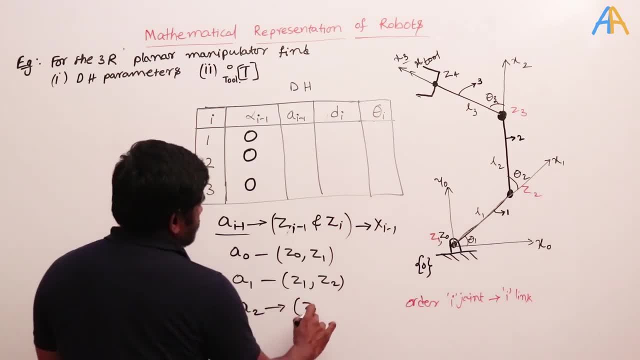 a 2 is nothing but z 2 and z 3. it is not angle, sorry, the distance between these two. okay, so here what is happening: the distance between z naught and z 1: both are coincident, so the distance between these two is zero, and the distance between z 1 and z 2 is nothing but the length. 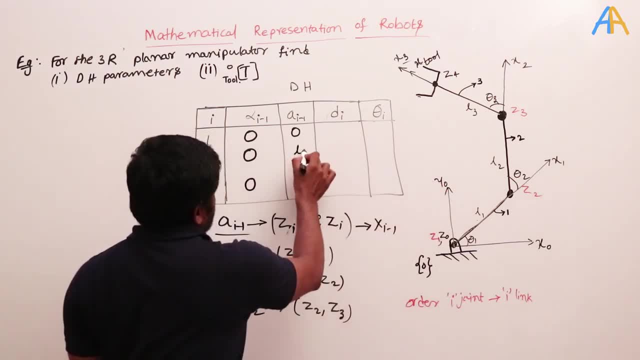 of the uh link. that is a l 1 here, and the distance between z 2 and z 3. this is the z 2 and that is the z 3. that is nothing but a l 2. okay, and now we need to find out. 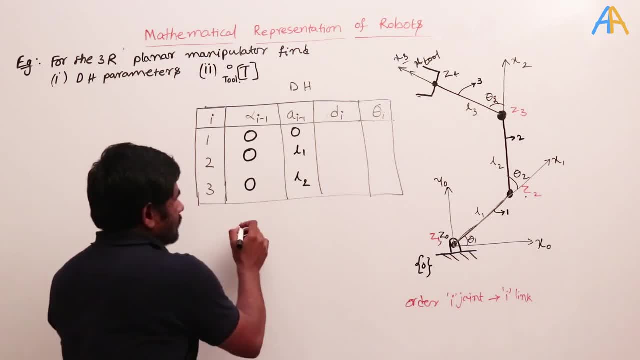 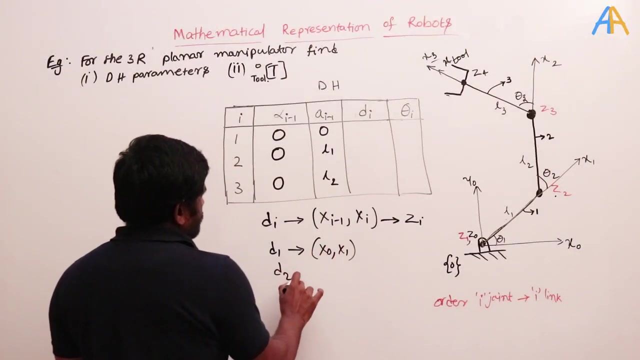 a, we need to find out di di. it is nothing but the distance between x, i minus 1 comma xi, between x, naught and x1, and for the d2 it is between x1. see, this is the first example. that's why i'm writing everything clearly, so after some time you should be able to figure it out, you know. 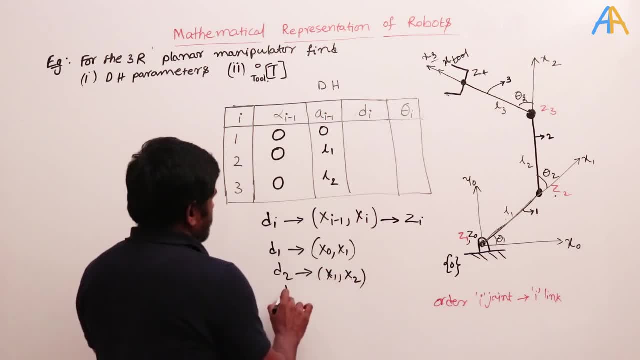 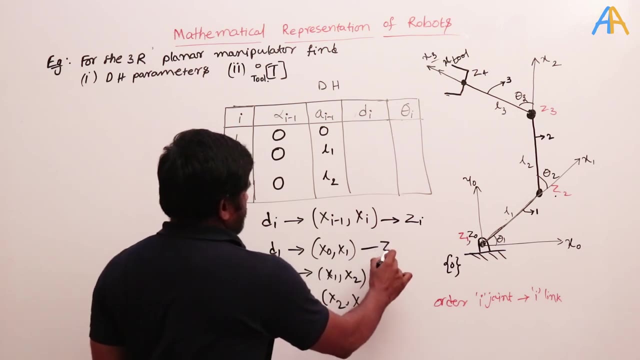 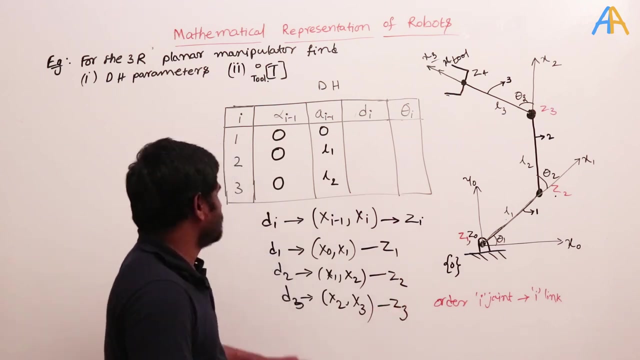 even without writing all this. so x2 and otherwise, if you feel, whenever you feel confusion, then it's better you write like this, then it will be easier under x2, comma, x3. okay, so here it is a yeah, you know, yeah, yeah, along the z1, z2 and along the z3. so what is the d1 value here? d1 is a distance. 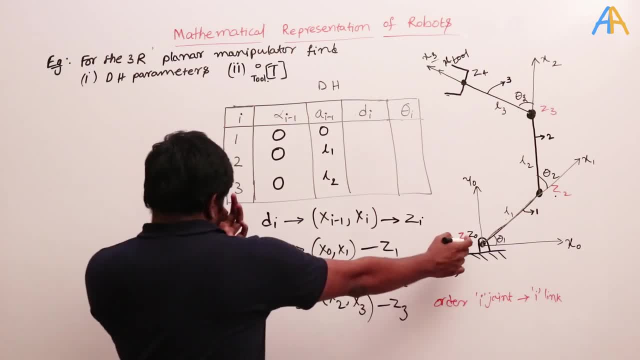 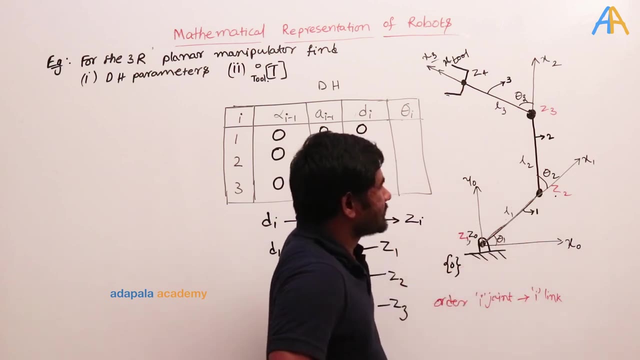 between x, naught and x1, but both are, you know, intersecting here. then the value is zero and d2. d2 is the distance between between x1 and x2. see here: x1 is this, and if i extend the x2 up to here, then both are intersecting at one point. so that means the. 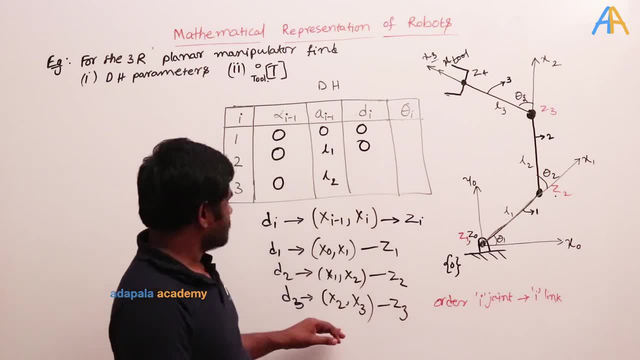 distance between these two is zero. again and again. what is the distance between x2 and x3? this is the x3 and that is the x2. again, both are intersecting at the point of z2. x is at the z2, so again it is. 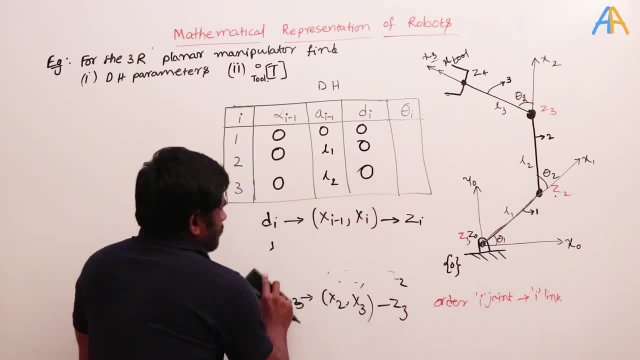 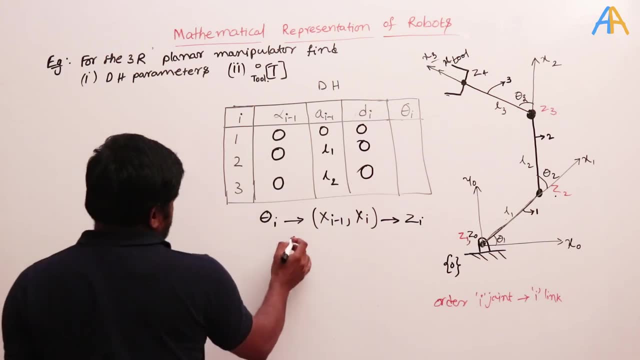 zero here and now. we need to find out. we need to find out: theta i, theta i again. this is the you know angle between a x i minus 1 and x. i rotated about the z i, so theta 1 is the angle between x 0 comma, x 1 and. 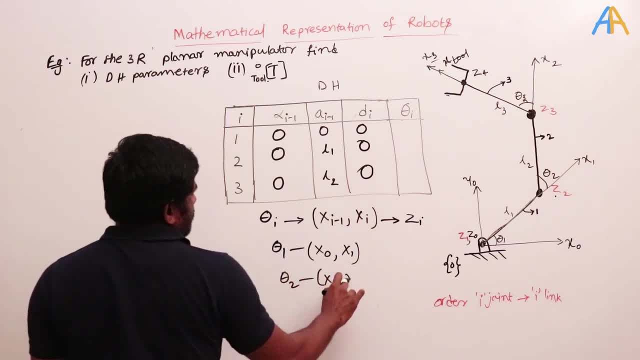 theta 2 is the angle between x 1 comma x 2, and theta 3 is the angle between x 1 comma x 2, and theta 3 is the angle between x2 comma x3. okay, so here what is happening? so what is the x naught? 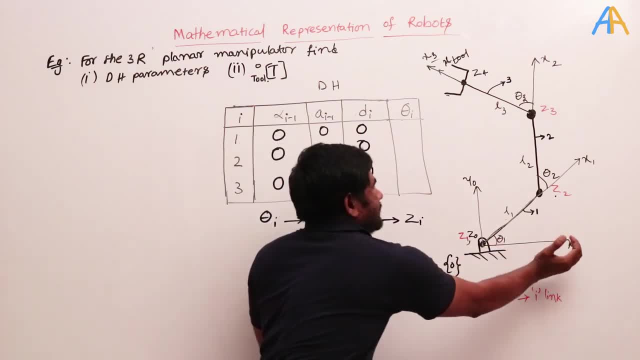 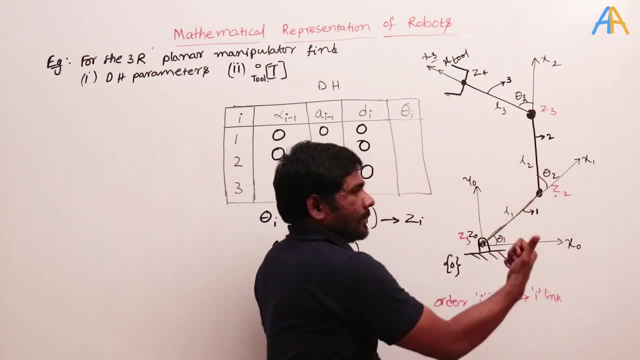 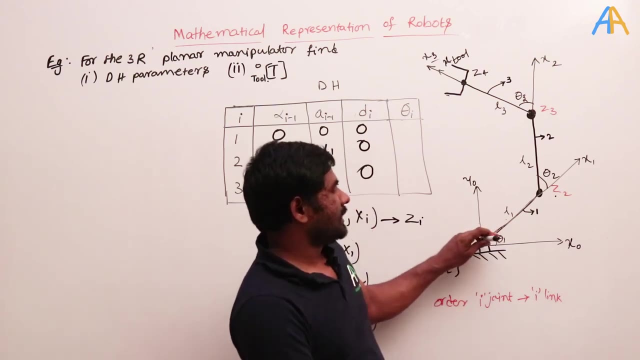 this is the x. Anderson, if i go from x naught to x, complain. it is the angle. this much angle i'm getting and the. you know, the thumb indicates the about which axis we are rotating here, about the z axis. here z axis is coming outward direction, so the thumb is in the 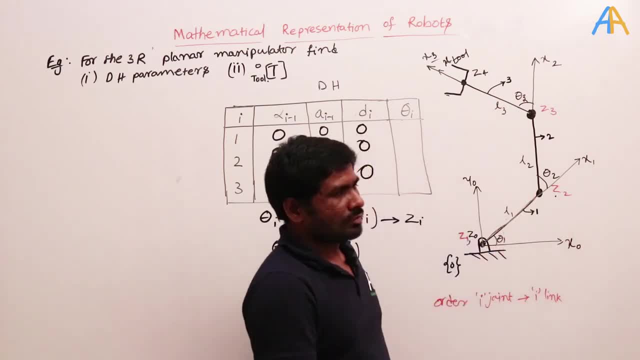 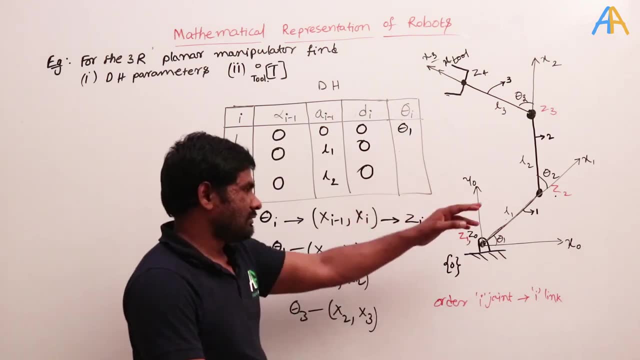 when I am going from x0 to x1- outward direction, so both are in the same direction. so the value of a theta 1 is a positive here. in this case, this is the theta 1. and in the same way, when I go for a, you know, x1 to the x2, like this: 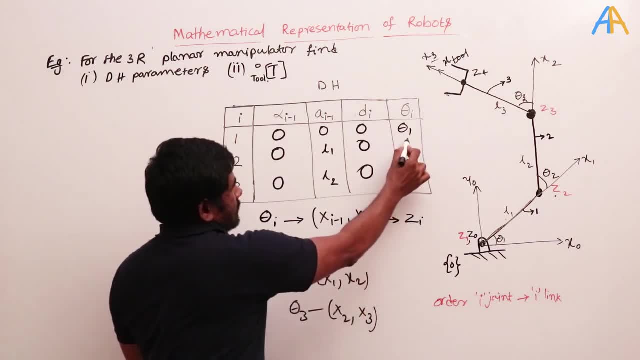 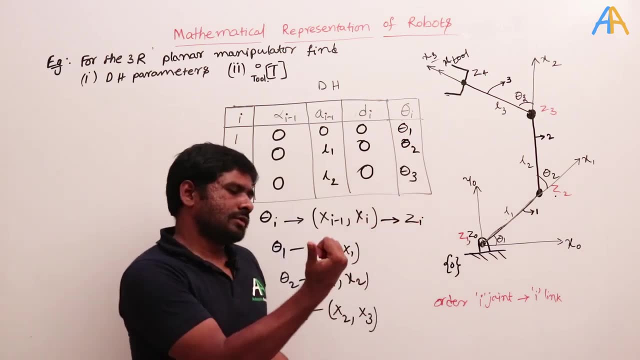 then again about the z2, then it is a theta 2. under the angle between x2 and x3 is the theta 3. you know, instead of all this pointing in the same direction, if it is an upward direction, then we need to put the negative sign here, as I. 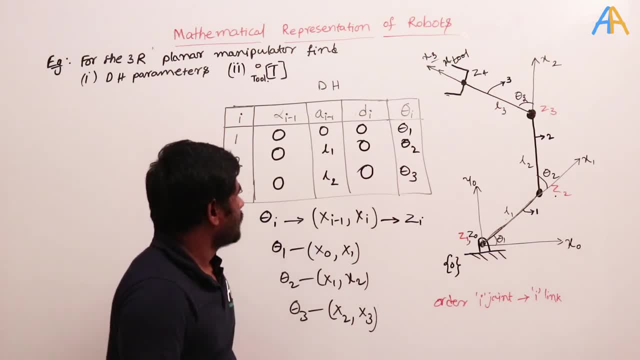 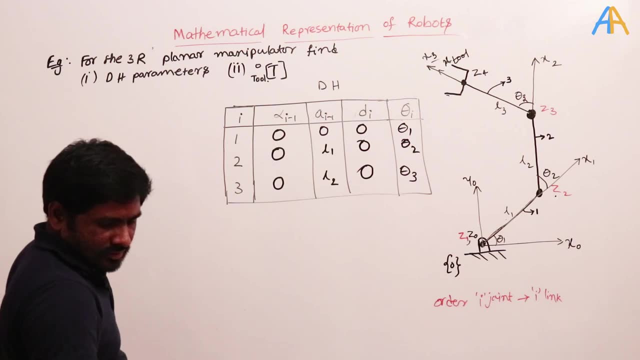 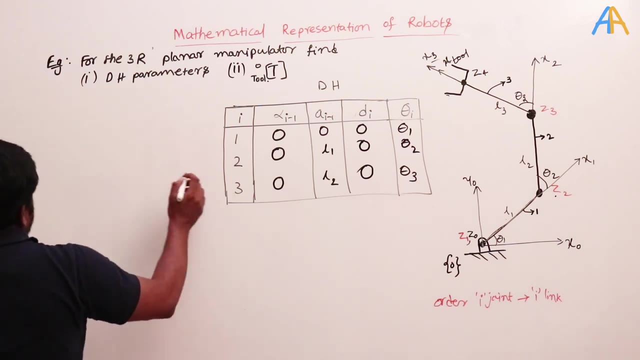 explained, you know previously. so, finally, this is how we need to find out the DH parameters. okay, after finding the DH parameters, then we need to write the. we need to write a transformation matrix. so, for the first transformation matrix, what is the first transformation matrix? I minus 1 to I, so if I substitute, I equal. 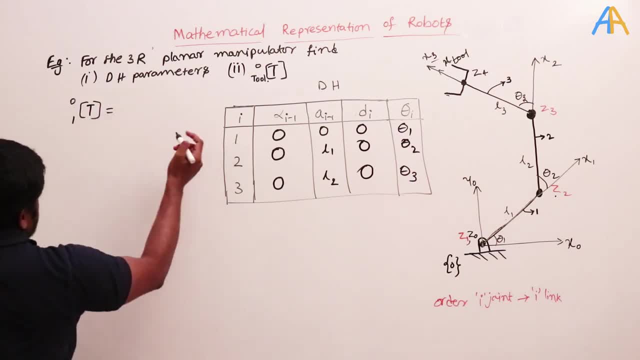 to 1, then it is equal to 1. so this is the first transformation matrix: I minus 1 to I. so if I substitute I equal to 1, then it will become 0 to 1. for the first one, 0 to 1 and either. you can remember that. 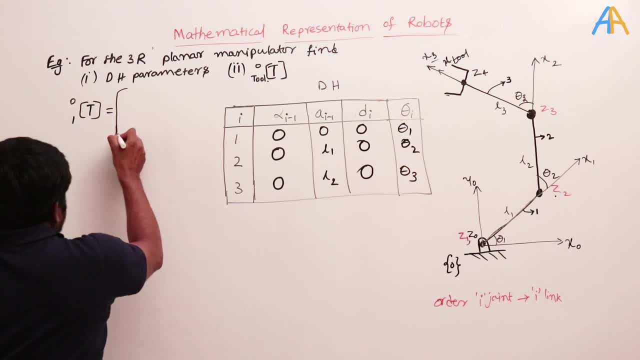 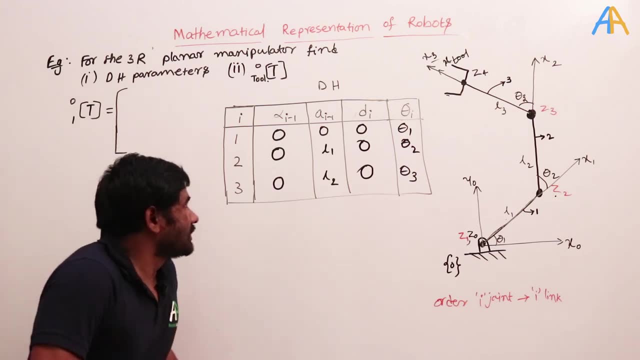 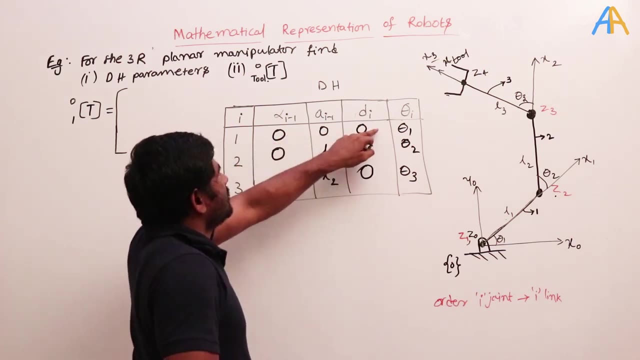 formula, final formula that we derived, or by using little bit common sense here, even without remembering that we can write the transformation matrices here. what is that that? for the first row, what is the value? alpha is 0, a is 0, d is 0. only theta is there under this. theta is around z axis, this is around z axis, and 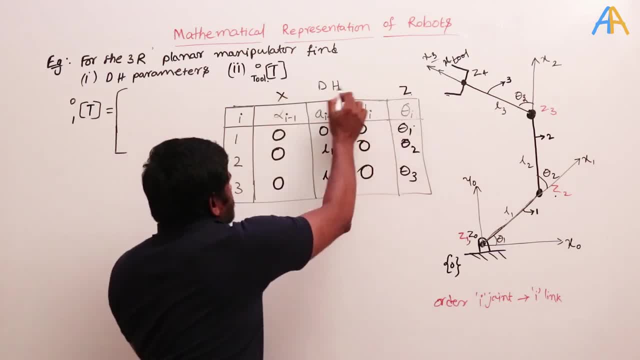 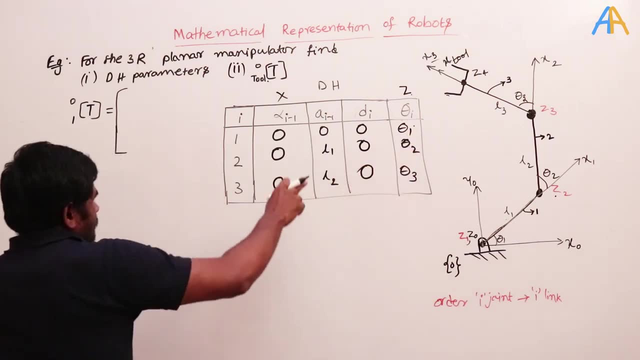 this is about x axis. this is about Jordan. this is about x axis. okay, so only there is a rotation about the z axis. so here I will write this as a C, theta C, T, C, 1, C, 1 means cos, theta 1, 1 for theta 1 and minus a yes 1, yes 1, C 1, 0, 0, 0, 0 here. 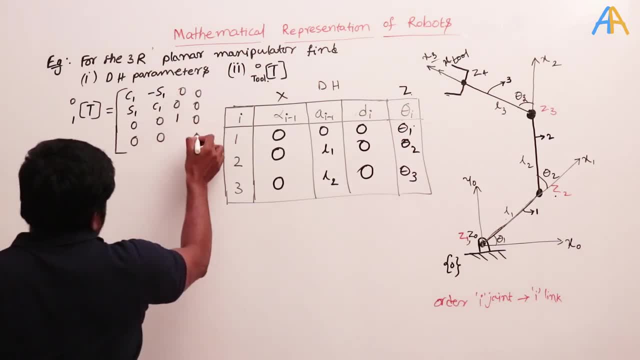 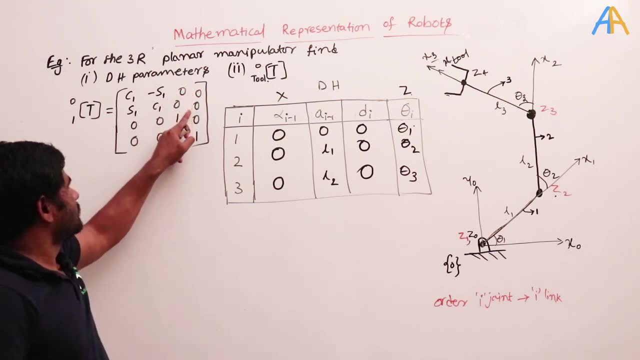 1, 0, 0, 0, 0, 0, 1 0. why? because here there is a no translation. this last column is a 0, except this one. because there is no translation. okay, in the same way I will write a transformation matrix. where the would link to that is I minus 1 to the I. 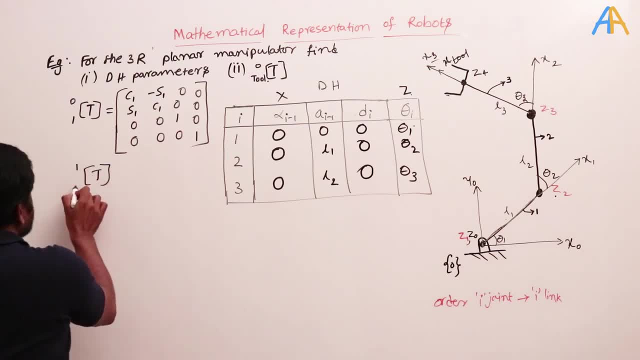 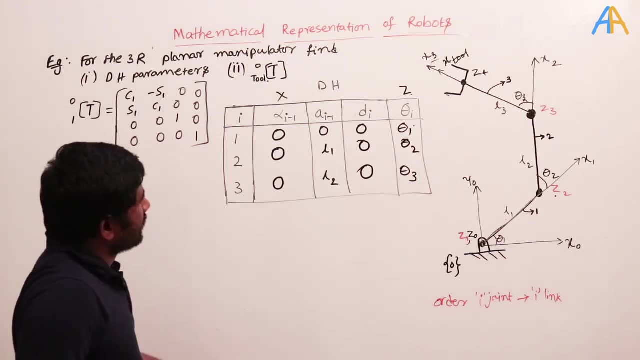 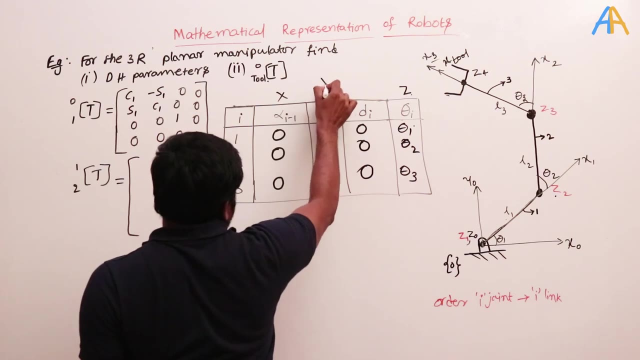 if I substitute I equal to 2, then it will become 1 to 2, 1 to 2 again. here, we will observe. you know, here, when I observe what is happening, there is a, you know, there is a. see, this movement is a along the x. 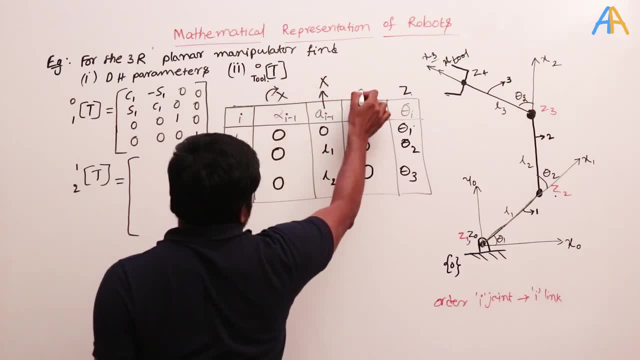 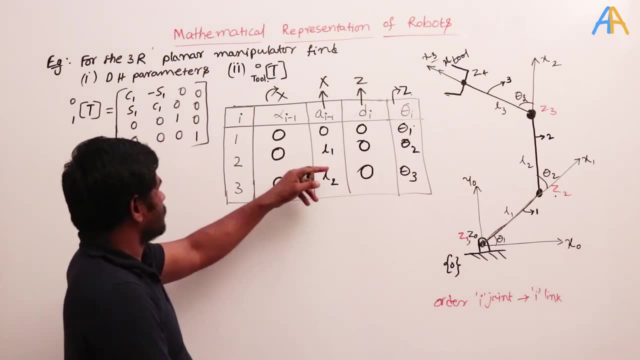 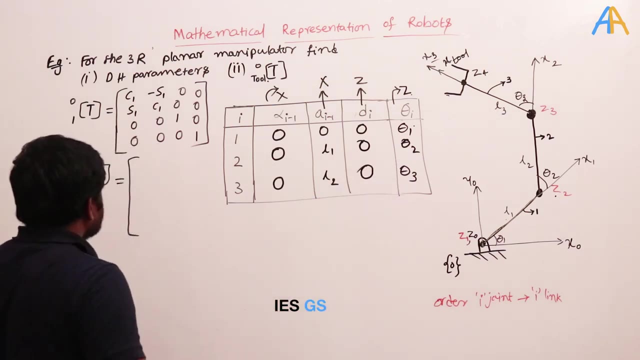 axis under. this is the about, this is a about and this is the along the z axis and this is the amount. okay, so you need to remember this. so there is a translation about the x axis. under there is a rotation about the z axis. only these two are there. so in that case, you know, only here, in case of a x coordinate. 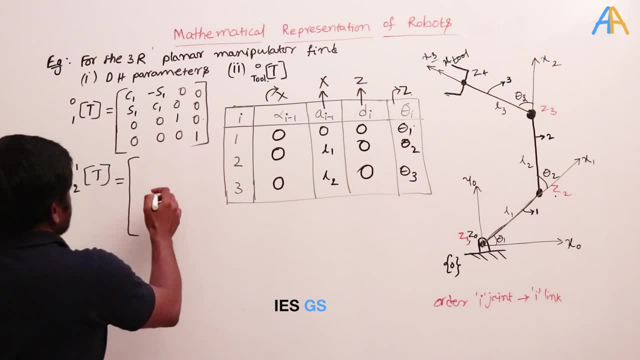 I substitute l1. okay, then it is easier. so here again, the rotation is about the z axis. whenever the rotation is about the z axis, again here c2 minus s2, s2, c2, 0, 0, 0, 0. again here 1 and again 0. 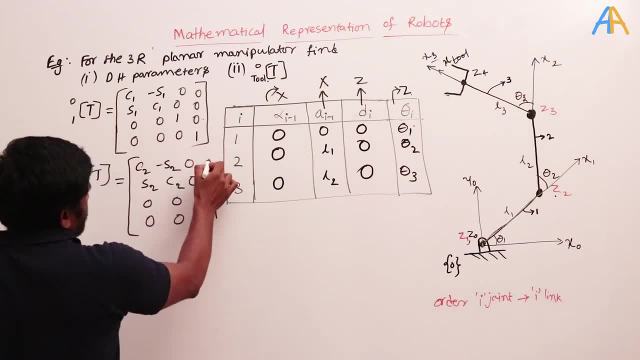 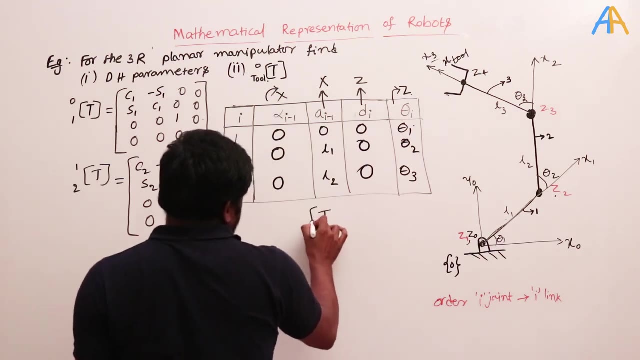 1, 0, 0, 0. and here i will write l1 and 0. why? what is the l1 here? this is the translation in the x direction. okay, then here i will write the t, you know, 2 comma 3, 2 comma 3, again the same process. 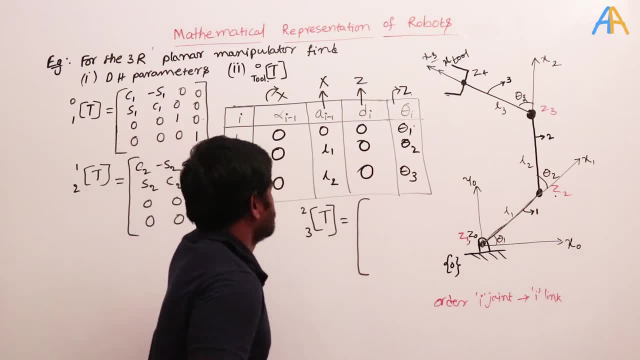 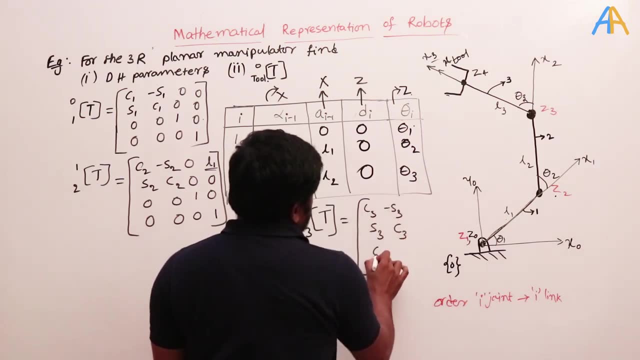 you know, for the link 2 and 3, same thing. so i will simply write a c3 minus s3, s3, c3, 0 0 0 0. again 1 0 0 0. here and here, here one, and here i need to write l2, l2 0 0, l2 0 0. okay, this is, that is what we need to write here. 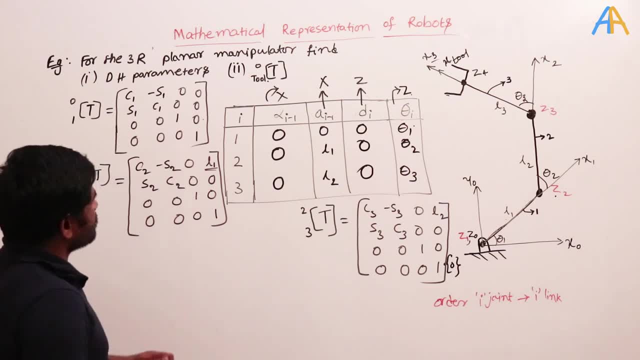 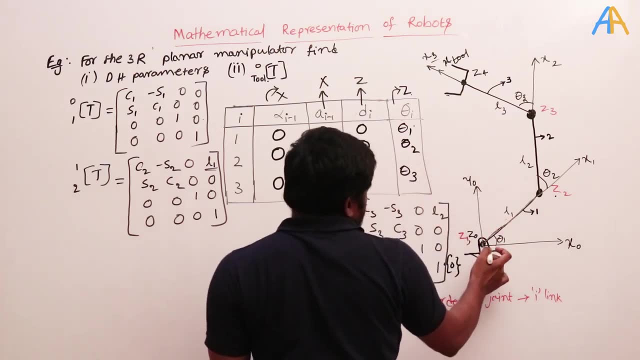 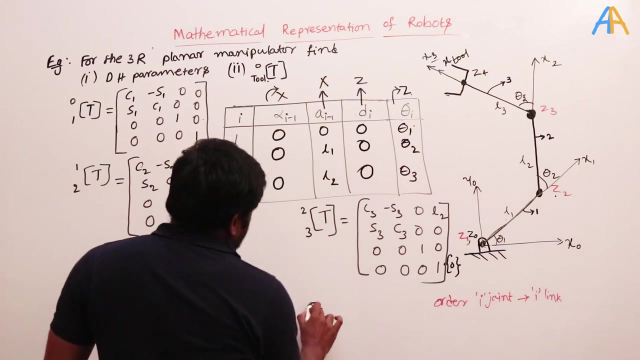 and here i have written. you know, dh parameter is a dh parameters. actually, the dh parameter table has taken me from here to here, from here to here up to the, this link 3, from here to here. i need to travel, so i will. i will write here one more thing: what is that t from the link 3 to the tool tool. 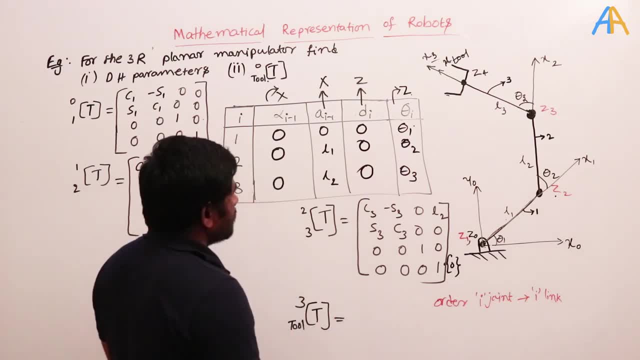 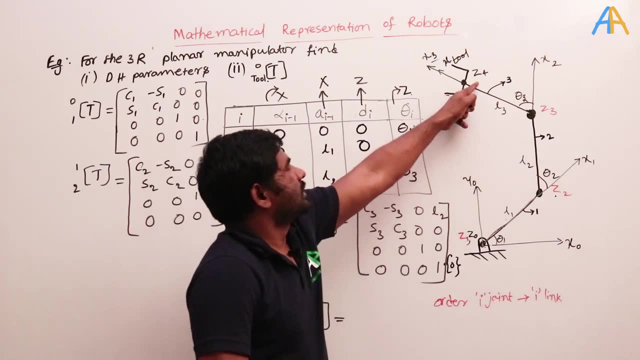 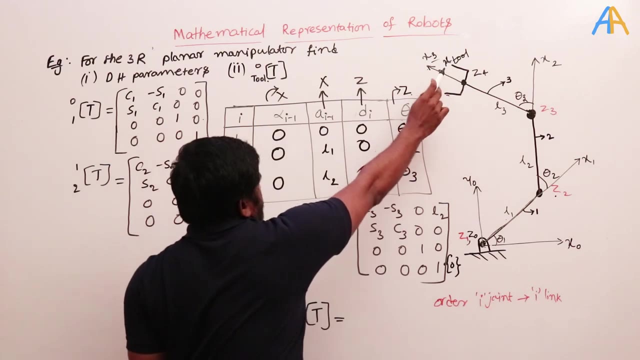 is at the end. okay, this is. i need to write here what is happening. the coordinate system that i have chosen is a. the coordinate system that is i have chosen, that is a z4, is exactly similar to the z3. that means there is no orientation. why? because at x3 is coincident with the x tool. okay, 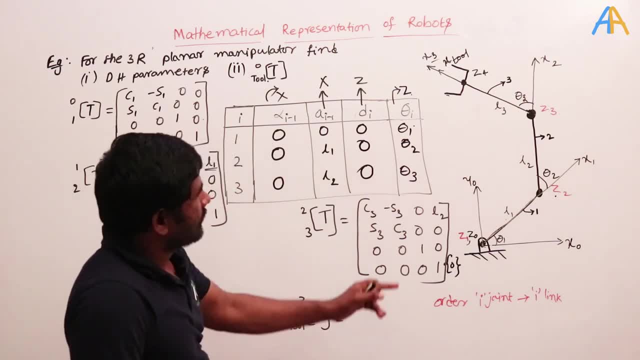 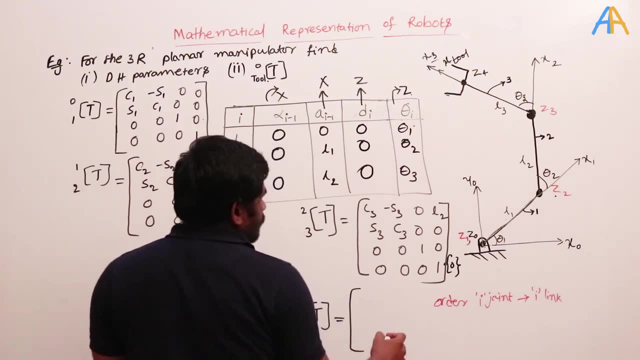 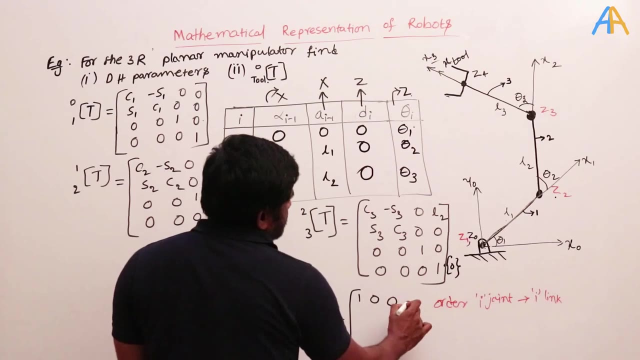 but only thing is it is a translating error along the x axis. it is only translating along the x axis, okay. that means when there is no rotation, then it is a identity matrix, okay. and it is translating along the x-axis. that means i will write here l3, but the distance is l3 from here. 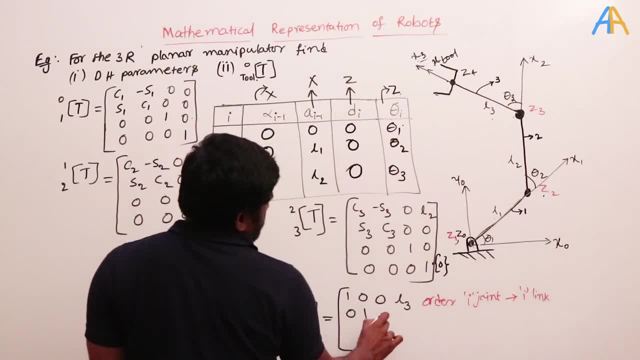 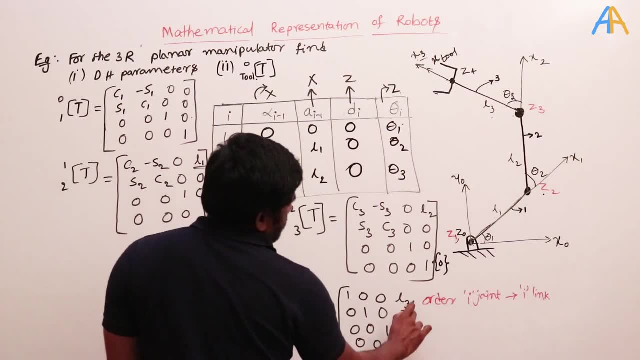 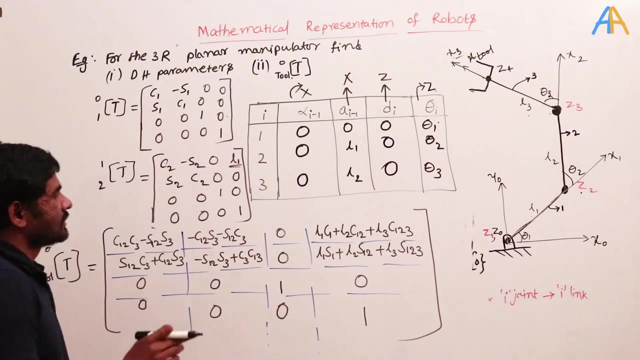 to here, along the x-axis, the x axis. so remaining is the identity matrix. so here, this is the one we will get: 0, 0, 0, 1. this is the matrix. so finally, if i want to get the final matrix, what is after a simplification, you will 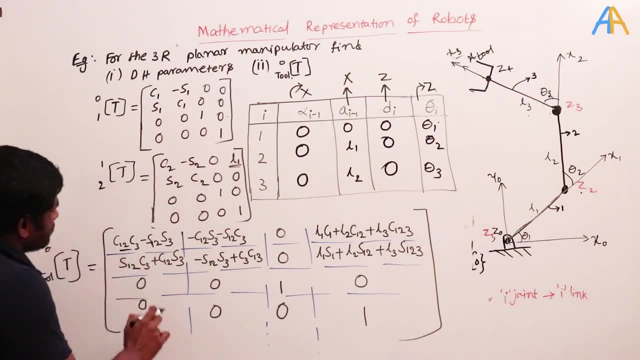 get finally this matrix here. what is the c 1, 2? c 1, 2 is nothing but a cos. theta 1 plus theta 2, okay. and s 1, 2 means sin of theta 1 plus theta 2. if i write c 1, 2, 3, then that means cos of. 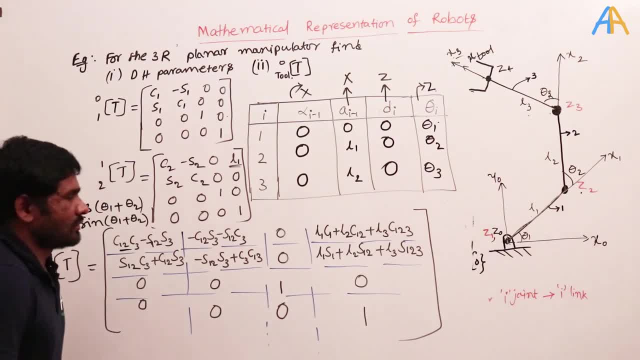 theta 1 plus theta 2 plus theta 3. that is the meaning. okay, no doubt you don't get confused. and when you are writing this in the examination now, you clearly state that c for cos and c, 1 for cos. theta 1, c 1, 2 for cos of theta 1 plus theta 2.